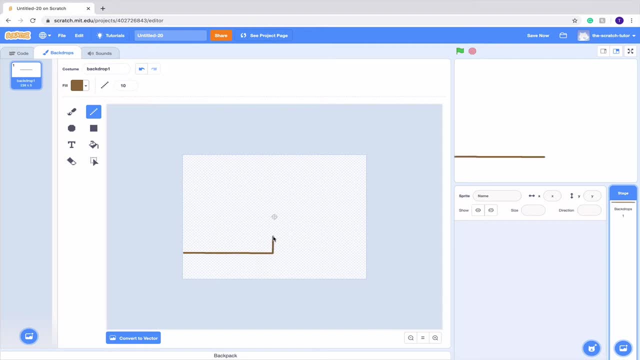 Say: This is just the regular floor here, Then I'm going to start the stairs like this, I'm going to make it go all the way up here and then it'll end right here. So, now that we have this, we want to create our person. 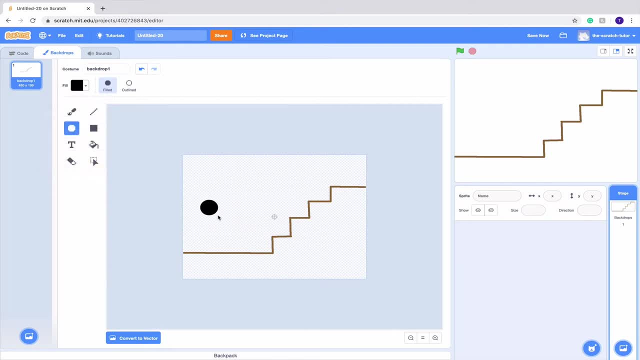 Mine's going to be really simple, just a stick figure. It's not going to have any facial expressions. There's our circle. I'm just going to make him have arms and legs. So we have our very basic area. Now what we want to do is duplicate it. 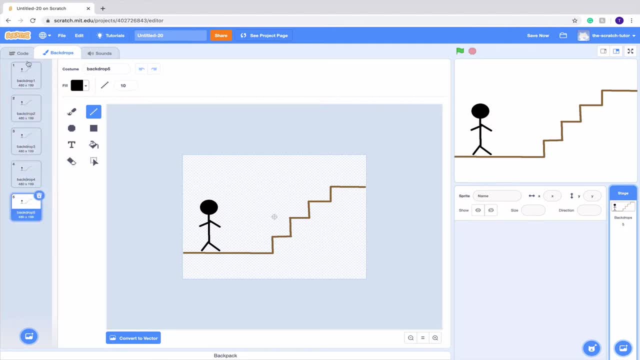 We're going to duplicate it, just maybe five times, for right now. Actually, no, We're just going to duplicate it once and we are going to take this move tool and we're going to want to select it, Move him over just a little bit and then make his arms and legs move. 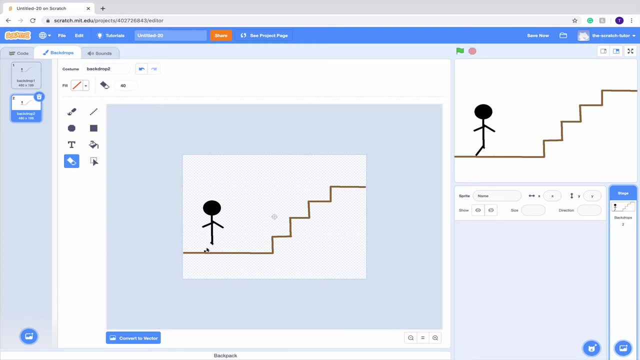 So I'm just going to erase his legs and his arms and then we're going to make it so it's different, So it looks like he's walking. So we have this. I'm going to make maybe this one a bit shorter and this one extend out a little bit. 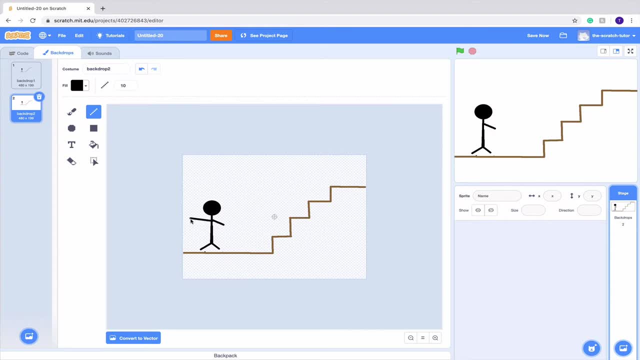 and then this arm down and this arm, like that, So it goes from here to here. Then I'm going to duplicate this one and I'm going to repeat the process. I'm going to select him, I'm going to shift him over a bit. 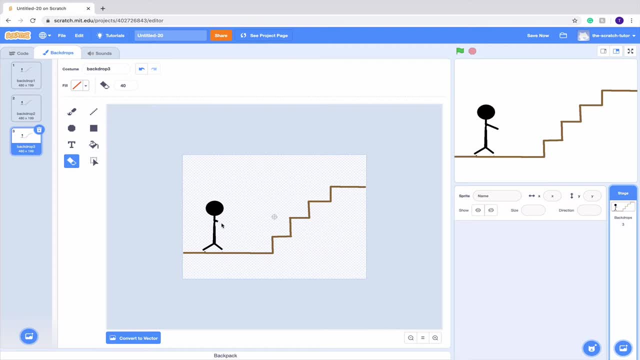 Then I'm going to change his arms and legs, Make it look like he's moving. So we just have his body here. I'm going to get the color we've been using and let's make this arm still get a little shorter. 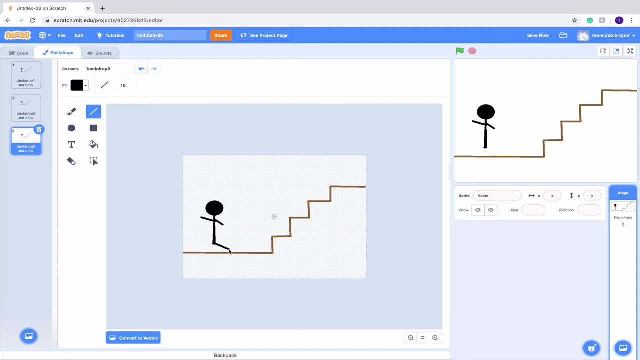 and this go here And this leg will extend more and this leg will stay like that, So he starts off here, He will start walking, And then we want to duplicate this one, of course, And we're just going to keep on repeating this process. 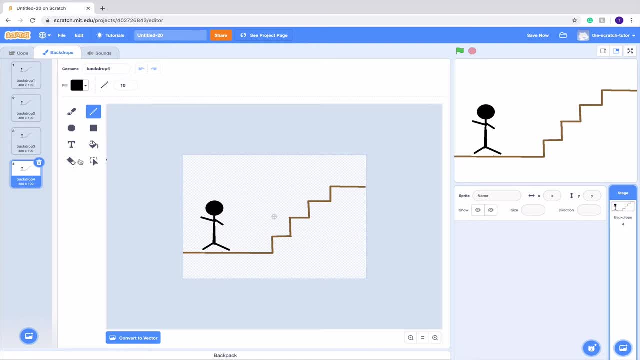 until we have him where we want him. So I'm going to just erase the arms and legs And I'm going to make him a new body right here And I'm just going to make this extend a bit, this extend a bit. 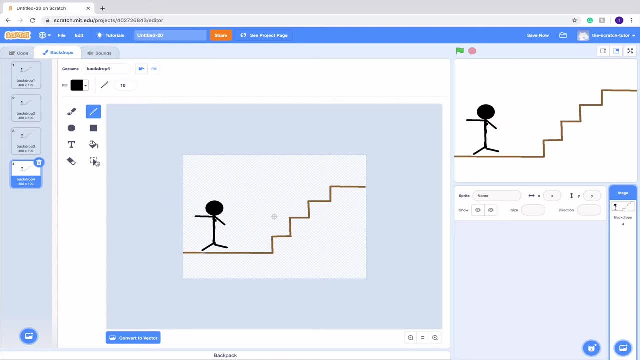 and this extend a bit. I'm just going to shift him over. So if we look at what we have, we have this backdrop. It goes to there, It goes to there, It keeps on walking. We're going to make his legs switch now. 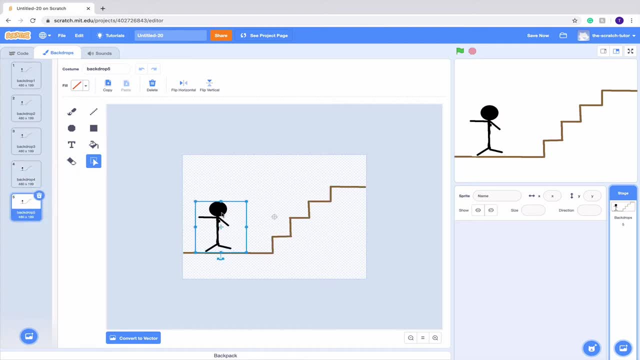 So I'm going to duplicate it, I'm going to select him, I'm going to shift him over. You can see, I selected a bit of the floor, so I'm going to Command-Z, which is undoing it, And I'm just going to go until I have his feet. 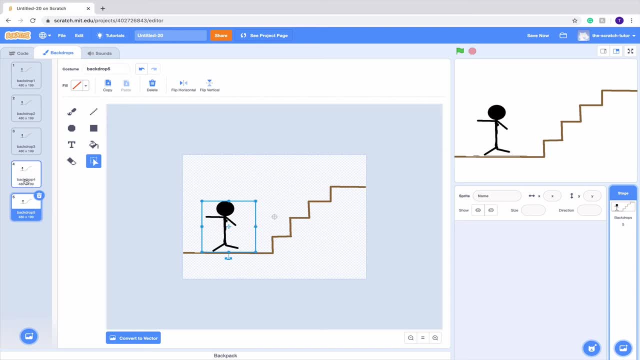 and not the floor this time. I'm going to shift him over right here And keep in mind, the more frames you do, the more smooth your animation is going to be. So I have this right here And I'm going to just switch up his legs and arms. 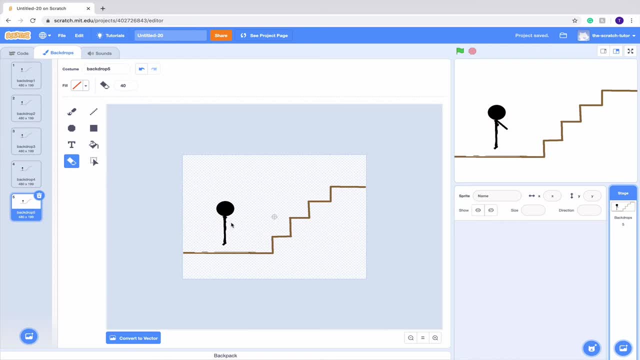 As usual. Okay, And I'm going to make his legs go back more now, And then his arms will also be doing the same. So it goes from here to here. We can see that his legs are not as long as they were before. 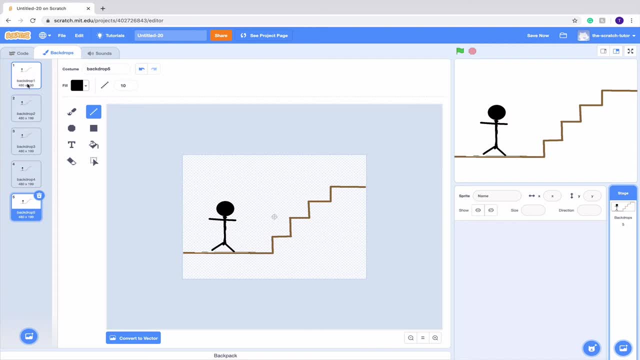 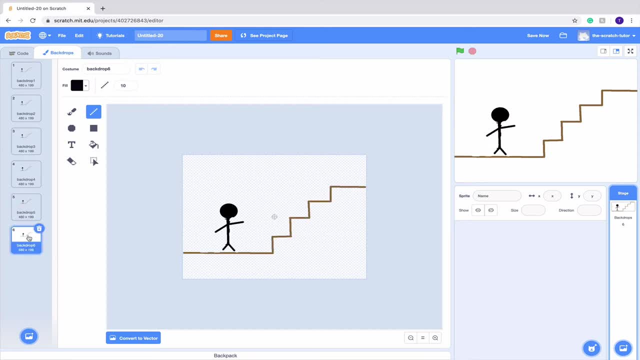 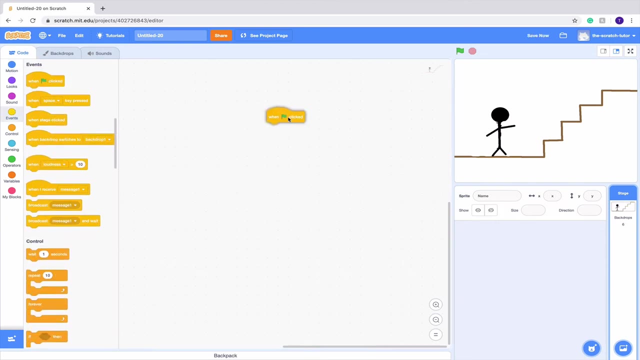 So he goes from here to here. His legs are a bit short still, So I'm going to just extend that, And now that I have just enough, we're going to go over the code of how to make it switch. So we're going to go to when green flag clicked. 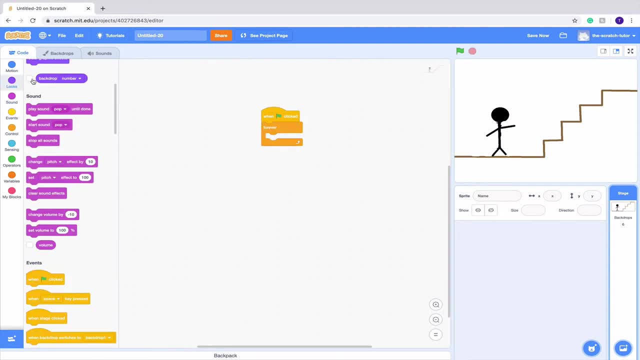 We're going to go to forever And then we're going to go to the look section And before the forever loop we want to switch backdrop to backdrop one which is the original backdrop, And then we want to drag in the next backdrop. 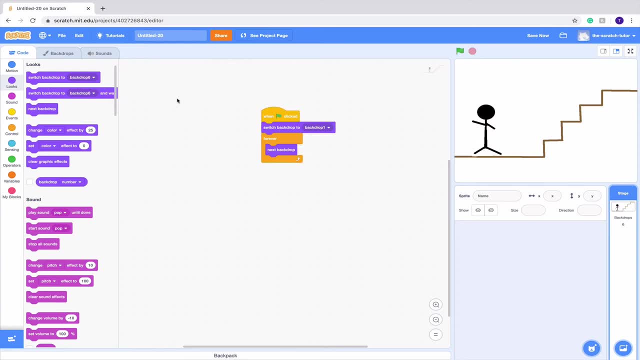 But if we see when we do that it moves super rapidly and we can't see a difference. So we want to go to our control section and drag in the weight block. So let's see what happens if we make it wait 0.1 seconds before changing. 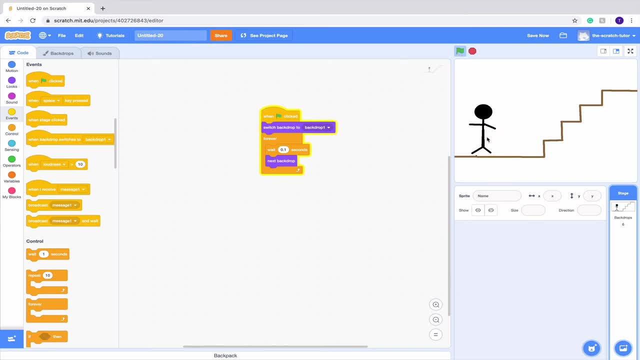 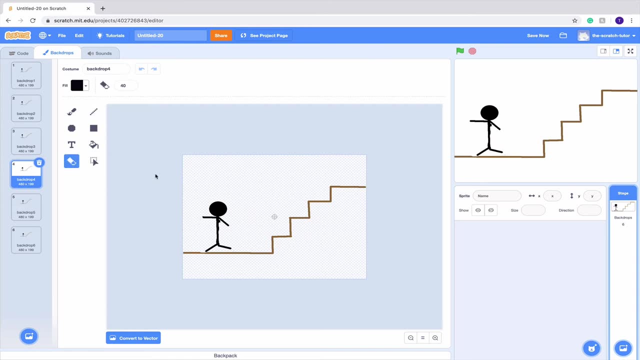 It goes like this: We can see he moves, We can see that arm gets a bit long there. And if we don't like that, let's go to where it's a bit long And let's just make it like that. And if we run it again, 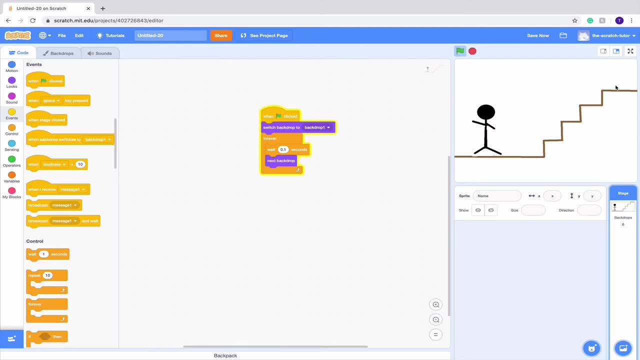 we can see that it doesn't get as long And we can see that he's slowly going to move up the stairs. If we don't like this and we want it to be just a bit quicker, we want to have it at 0.05.. 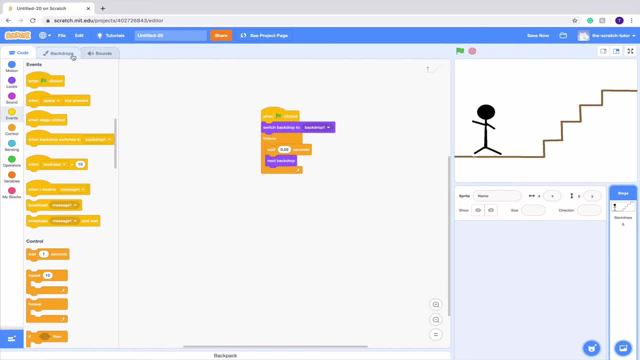 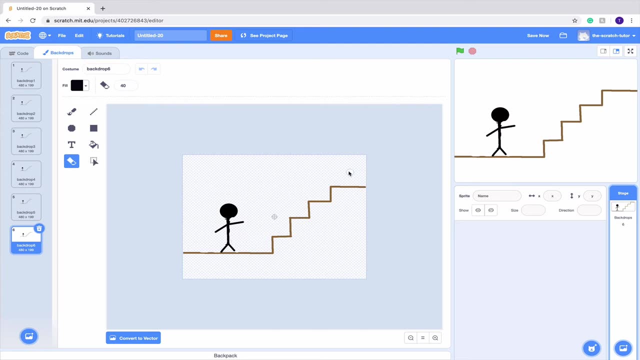 You can see he's moving faster And I kind of like that speed. So I'm just going to go and keep on creating more and more of these different stick figures going up the stairs until I've reached the top. right now I've completed about 11 different backdrops and if we check on, 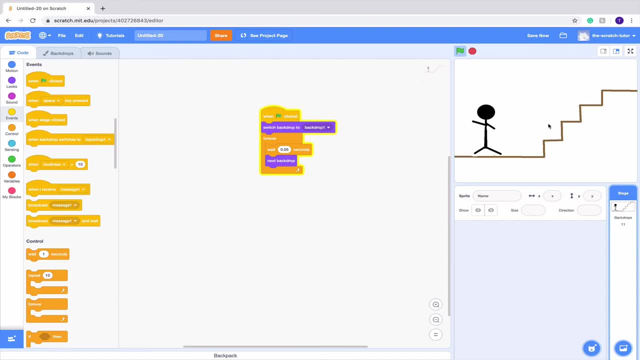 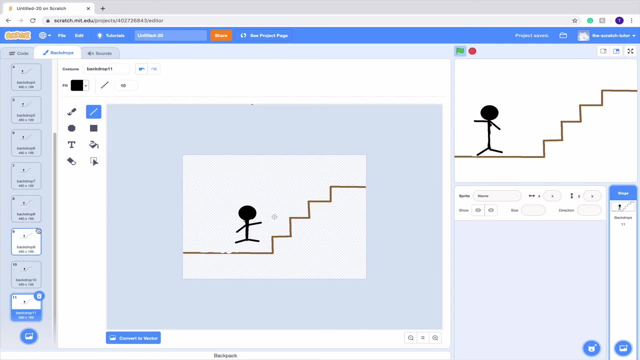 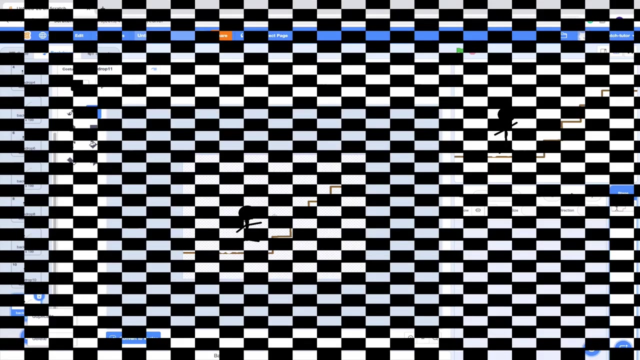 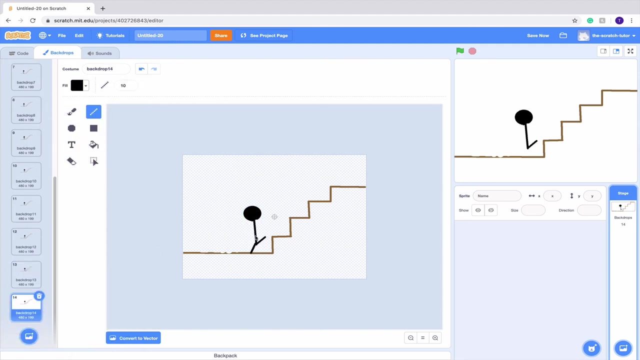 what I've done so far. we can see that he is moving and he's going to go up the stairs soon and I'm just going to keep on creating more and more and we are going to go into back into a time-lapse. you did about 20 more and we can see our characters is almost getting to the top. 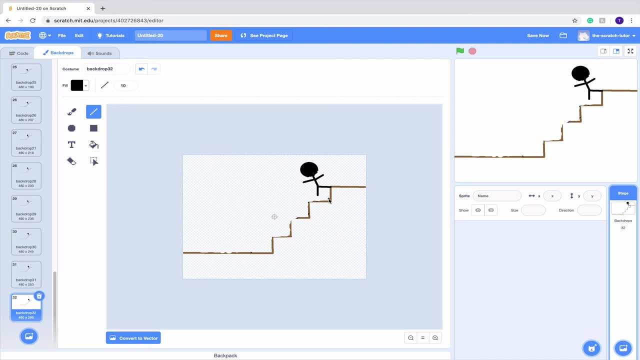 of the stairs, and for me, I'm going to try and make this an endless loop, so I'm going to make him, once he gets to the top of the stairs, fall down, and then he will just be keep on looping and looping forever and ever. so I'm going to keep on. 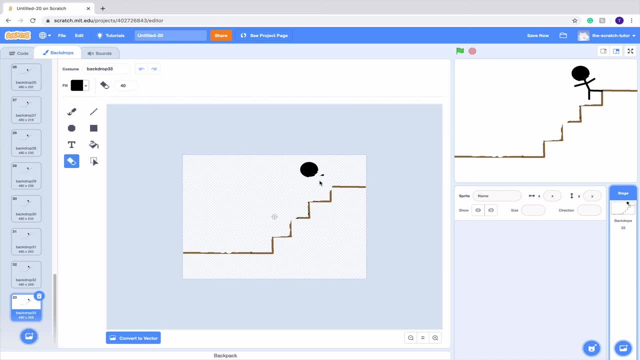 creating it until I get to the end point, you, you, you, you do. Thank you. So right now I finished all of my different slides and if you see here I made it, so he will. he fell down the stairs and there's this invisible force pushing him down, and then I made him morph. 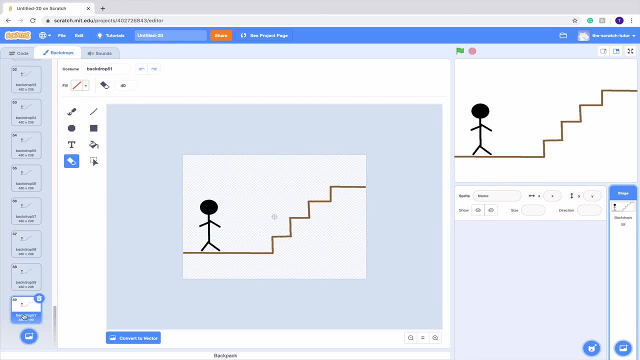 into the regular and then it starts off with the very first slide. you can do that easily by going to your first slide here and pressing duplicate, and then you can drag that all the way down to the bottom. So if we take a look at what I've created, you can see he goes and walks. 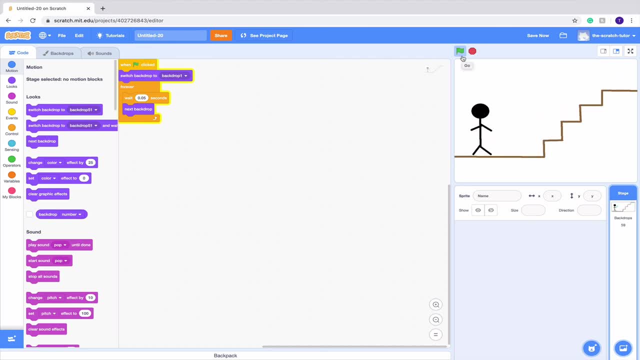 up the stairs one by one and then the force pushes him down and then it just keeps on looping over and over and over. and just an animation, really, really cool. So I hope you really enjoyed this video and if you learn something new, be sure to like and subscribe.